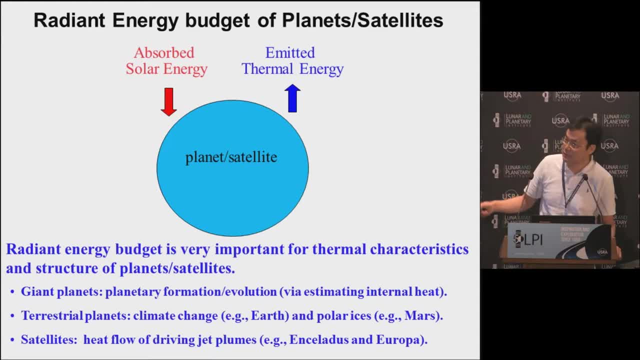 for planet or satellite You can see right here you can find, for whatever planet or satellite, it gets energy from sun And at the same time it gets energy from the atmosphere. So that's the third one. It radiates energy to space. So you have some balance on the top of the atmosphere. 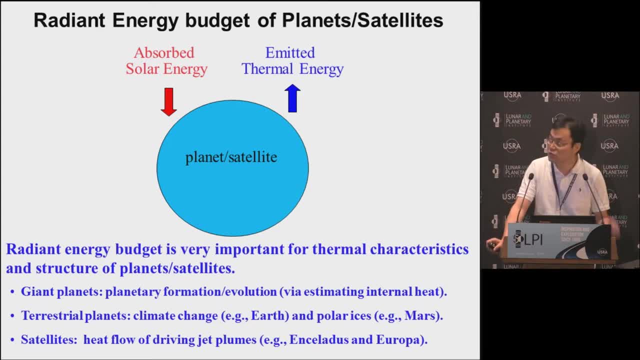 So, but anyway, for the terrestrial planets or satellites, only two energy sources. one is from sun, the other is the outgoing energy. So basically two energy sources that determine the energy budget. But for the giant planets that's different. There are one more energy. 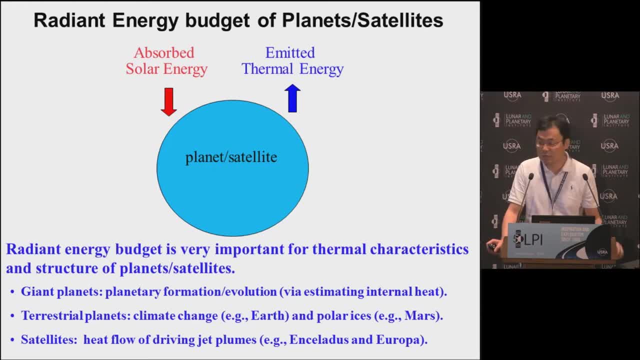 source from inside. we call internal heat. So internal heat is pretty important. It's very closely related to the planetary formation and evolution. In other words, internal heat can help us to understand the planetary formation and evolution For the terrestrial planets and satellites. radiant energy budget can help us to understand the climate change. 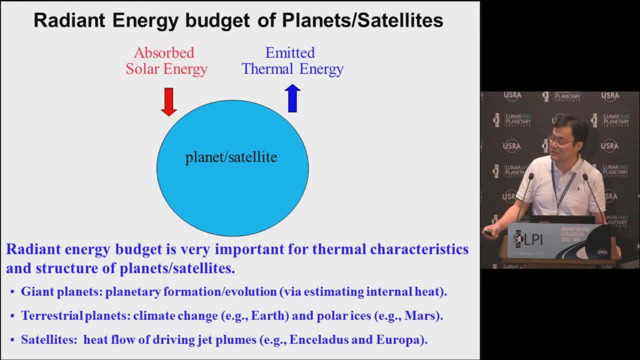 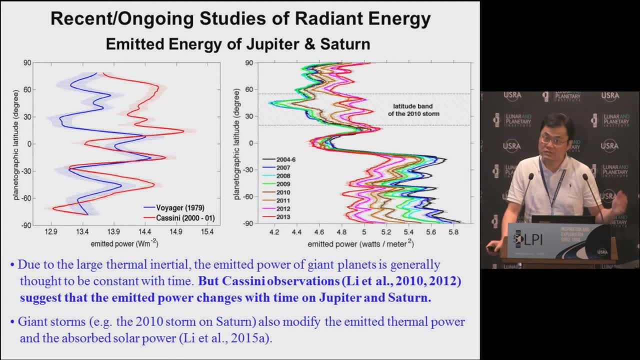 the polar ice, even the jet plumes on some satellites like the Enceladus and Europa. Okay, Right here I want to talk about some recent progress. You understand the energy spending, the radiant energy budgets of the planets. This slide shows the immediate power. 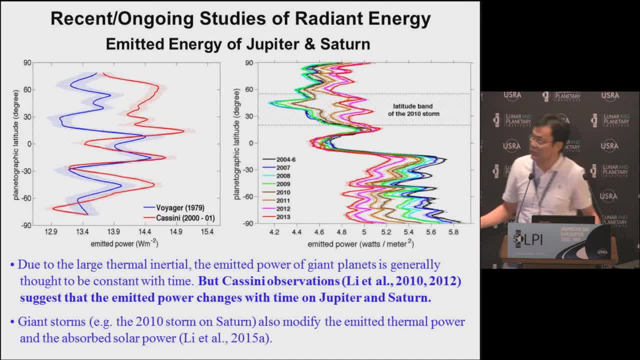 of Jupiter and Saturn. The left figure shows the immediate power of Jupiter. This direction is the immediate power. What you got? the reaction is the latitude. The blue curve, blue profile, is observation from Voyage. that's 1979.. The red line is observation from Cassini, that's. 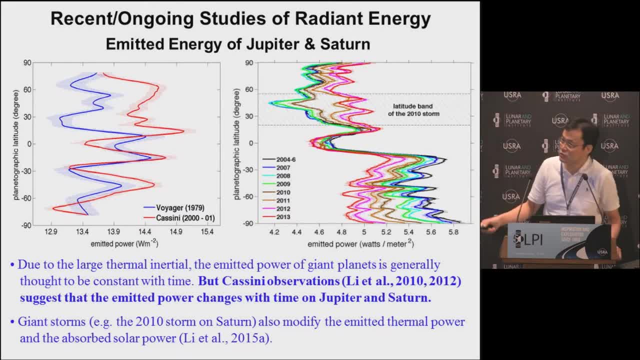 2000, 2001.. The comparison right here shows a very strong temporal variation from Voyage time to Cassini time. That's for Jupiter. This panel shows the immediate power of Saturn from 2004 to 2013,- roughly 10 years. Also, you can see very clear seasonal change in the two hemispheres. 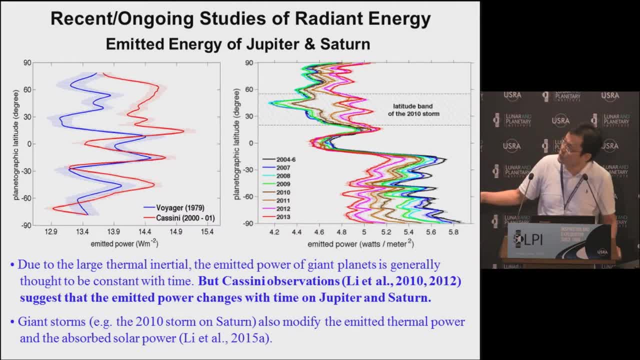 from 2004 to 2013.. Also, if you pay attention right here, median latitude is in the lower hemisphere. From 2010, this curve to 2011, that there was strong increase of immediate power on Saturn. Why? That's because 2010 giant storm happened in that year, So in other 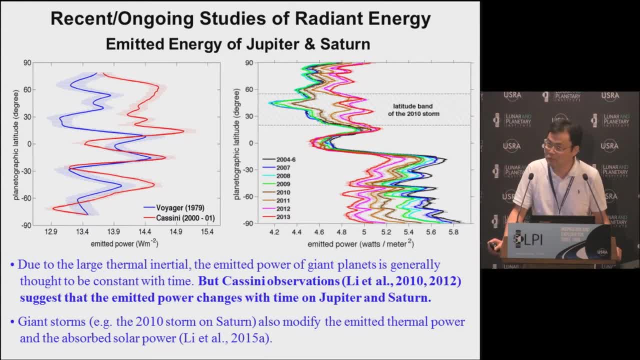 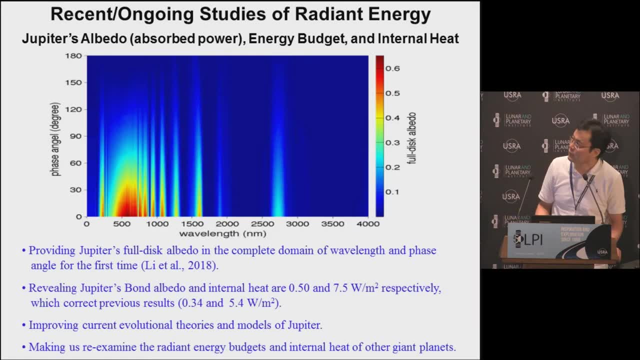 words. we think the giant storms are very important for the radiant energy budget on giant planets. Okay Here, immediate power. only the part of the sun changes, Because if we don't have energy because we're building with the, we look like the. 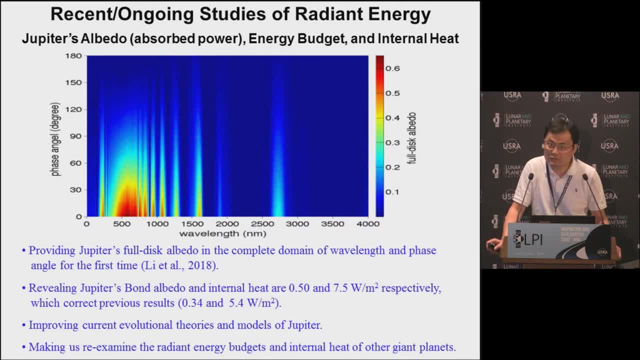 part of the story, because the radiant energy budget is determined by two energy sources. One is the outgoing energy, the other is absorbed solar energy. The absorbed solar energy is determined by albedo. Right here I show, right here is the solar disk, albedo of Jupiter, The two-dimensional. 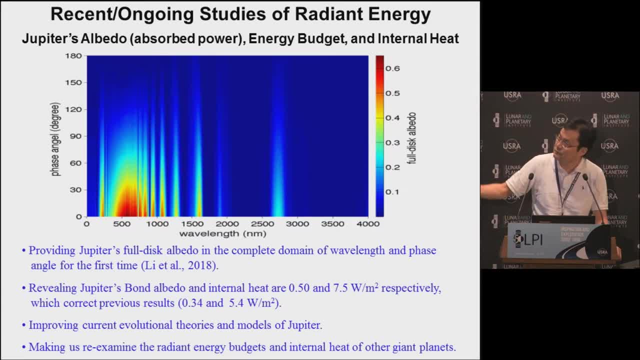 demand. one is the wavelength to this direction, other is the phase angle. So I think that's the first time we got this, because the Cassini observations are perfect, So we have the chance to get a two-dimensional albedo for Jupiter for the first time, Anyway. so you can find, based on the 2D. 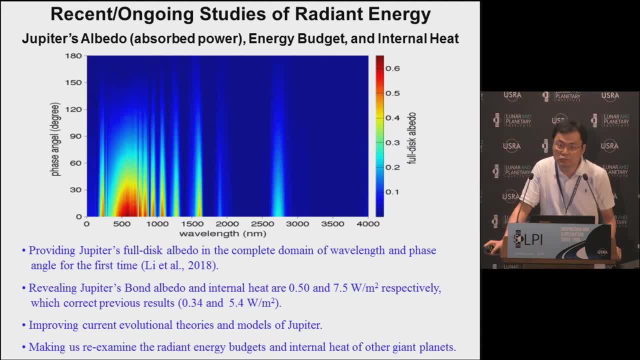 4D scale albedo. like this we can calculate the boundary albedo of Jupiter, which is 0.5, based on right here. Also we can calculate the internal heat for Jupiter. We got the value is 7.5 per meter squared. 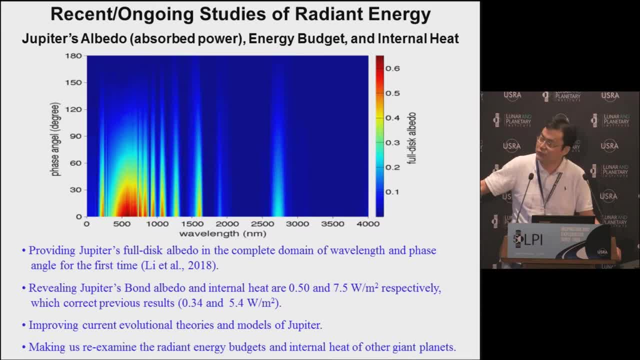 That's the new values. I put it right here. but if you compare the old values from the very limited observations, that's from Voyage and Pioneer, you can find a big difference. The reason is because I think the previous observations not that good: Pioneer, Voyage. 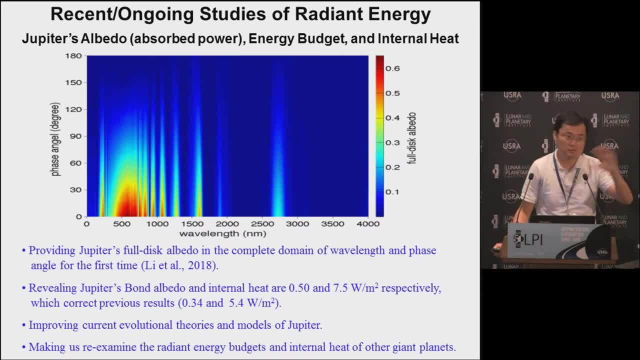 you know the phase angle. it's very limited. Also, the wavelength coverage is not perfect. So I think, in my opinion- I think actually we just published this paper on laser communications- Anyway, we think the new values right here are best results for Jupiter. Internal heat is pretty. 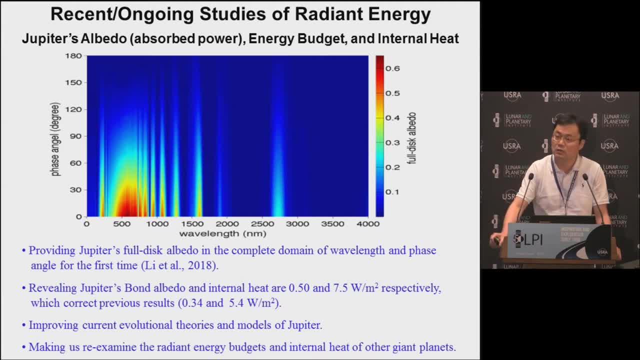 important for the giant planet, for the formation and evolution. So the new results right here make us to double check the models and theories of planetary formation and evolution for the giant planets. Also because right here we show the results for Jupiter. Jupiter results should suggest. 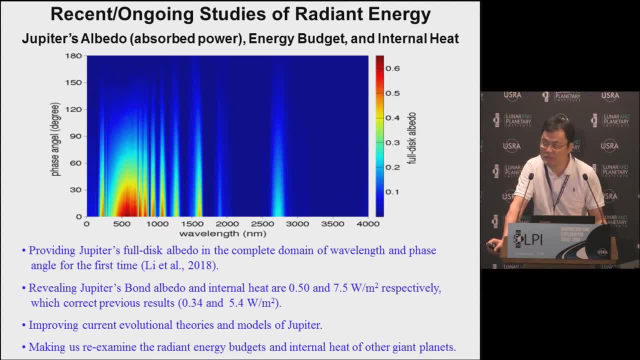 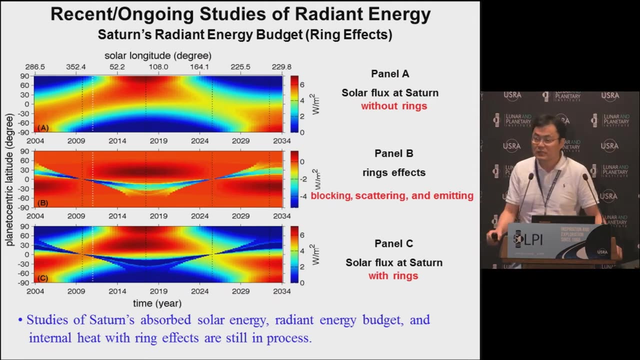 probably the previous measurements of the radiant energy budget and internal heat of giant planets are not correct, So we have to double check not only Jupiter, but also other three giant planets. That's the point. Okay, that's for Jupiter, Let's move to Saturn. Saturn is much more complicated. 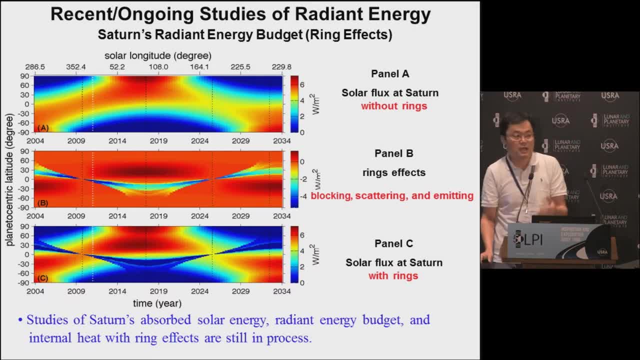 Why? Because the ring effects, The rings can reflect, block, even re-emit radiance, so make the radiant energy budget very complicated. But anyway, we got some progress. Here is, you know, we have a ring, very complicated ring model Based on that. 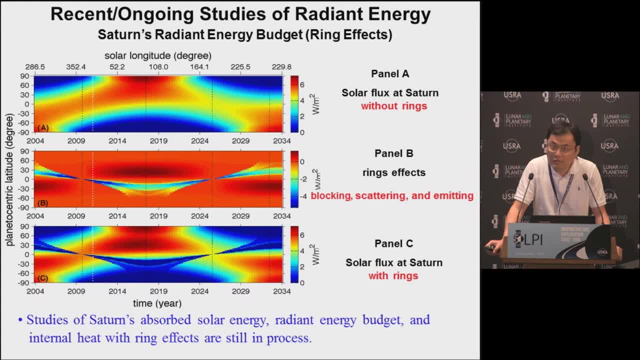 we have, you know, calculated the solar flux on Saturn. You know the time goes this way: the latitude goes with the vertical direction, So the top panel shows the solar flux and Saturn, without the rings. That's pretty easy to calculate. But anyway, the second way is very complicated. 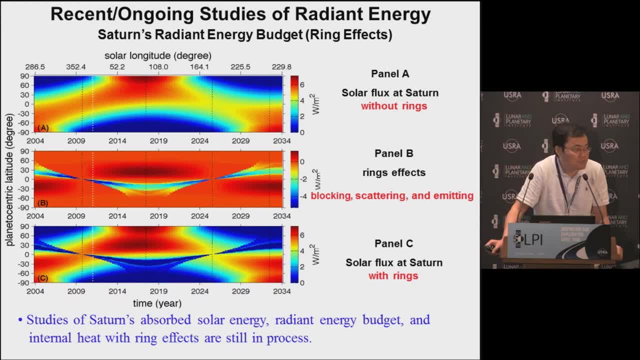 So blocking scattering, emitting. we have a very fancy formula to calculate, But anyway, we've basically finished it. Use the ring effects in the second panel. So we put that together. we have the last one for the solar flux and Saturn with ring effects. 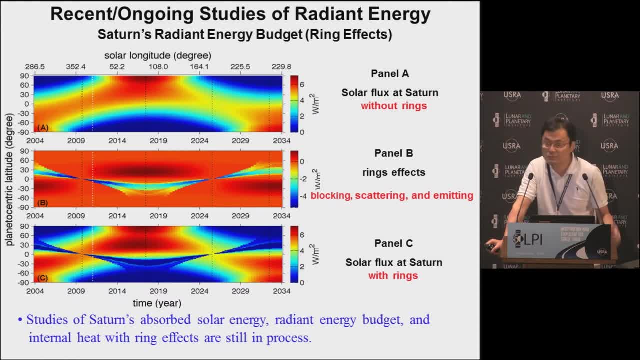 So that's pretty important. So based on this, also based on the Cassini observations, we can calculate the absorbed solar radiance. Then we can finish the story of a radiant energy budget. so we say that saturn Brad is the second largest solar radiation on earth. 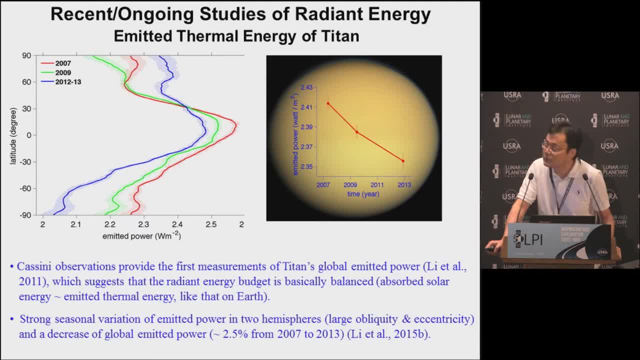 So basically what we will do is try to calculate the absorption, absorption rate of the atom and its enduring forces. So well, we've done that. but theoretically what would process is we can do actually thermal horoscope inv, että to calculate theuvo center of the calculations. 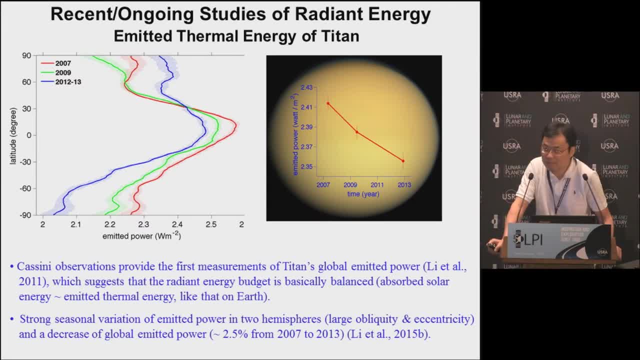 So year for titan actually is 30 years. it's pretty long. right here is the seasonal change, but anyway. also we combine the new observation of immediate power right here with the old observation of the absorbed solar radiance. then we conclude. you know, we think the radiant energy budget of a titan. 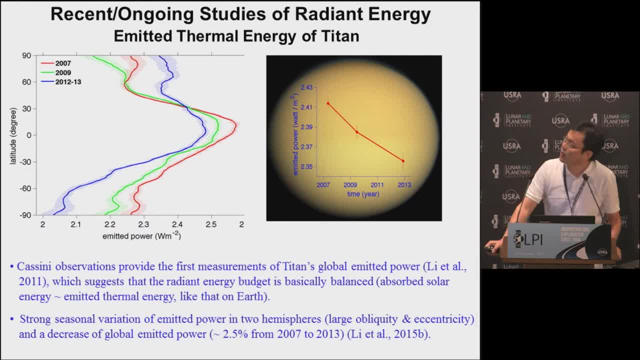 is basically balanced. okay, the also we. this panel shows the global average immediate power of a titan from year to year. so basically from 2007 to 2013. you can find the global average immediate power decreased with time, so roughly decreased 2.5 percent from 2007 to 2013.. immediate power. 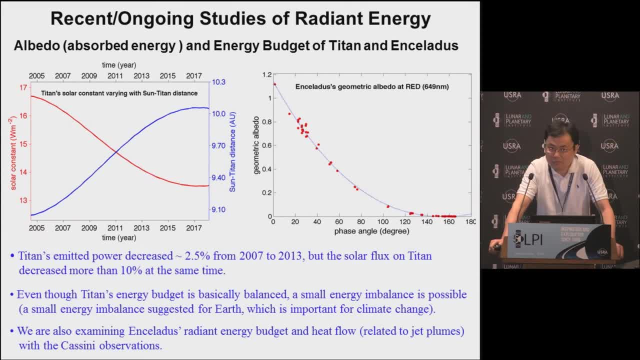 decreased on saturn from 2007 to 2013 and same time, solar flux decreased more than 10 percent from 2007 to 2013.. this figure shows, you know, the distance between titan and sun increased, so the solar flux decreased more than 10 percent. that means it's still possible a small energy. 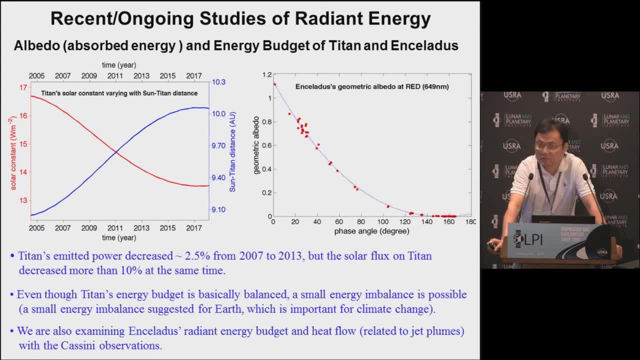 imbalance happens over there on titan even. you know we could, we think the roughly, you know the energy budget is roughly balanced but still possible a small energy imbalance. the reason is because recently a small energy imbalance suggested for earth also. people think the small energy imbalance probably is very important for climate change, for global warming, right here with we. 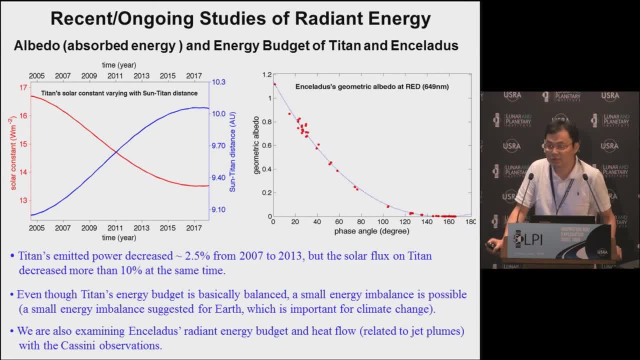 suggest it's also possible for titan, a small energy imbalance. we still double check because we have to calculate the immediate power, also calculate the absorbed solar radiance. then we can get the whole story. that's what that's for titan. we're still working on that. this is for enceladus. in recent years 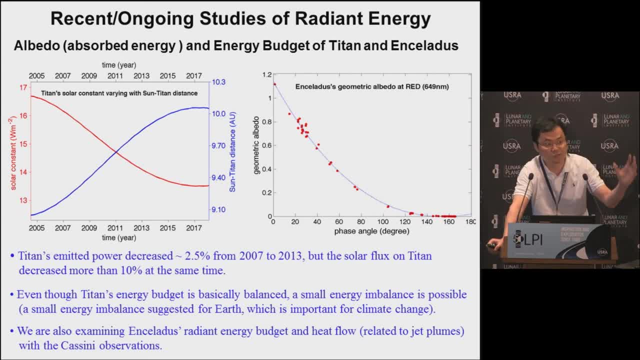 enceladus is pretty hot because we discovered the jet plumes in the source pole. right here we calculate the albedo four disc albedo based on casino observations. right here, just for the red wavelength, your first angle go this way. that's the geometry albedo. so we basically finished, okay. two. 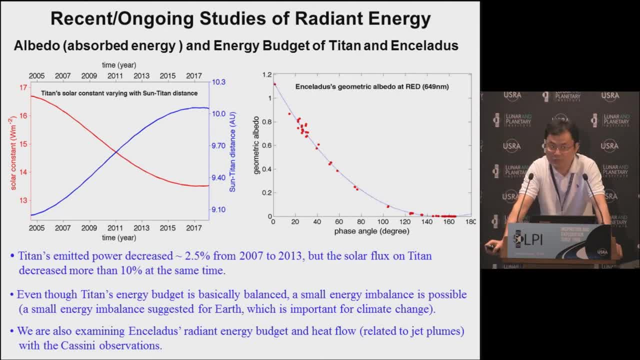 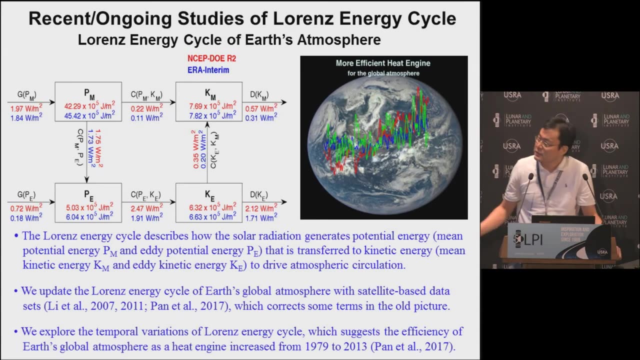 minutes. right, okay, we basically finished the calculation of the immediate power for enceladus. we still working on the outgoing energy. then you can finish the whole story. okay, right, here is the second topic is the lawrence- uh lawrence energy cycle of earth and mars. so basically, the lawrence energy cycle provides 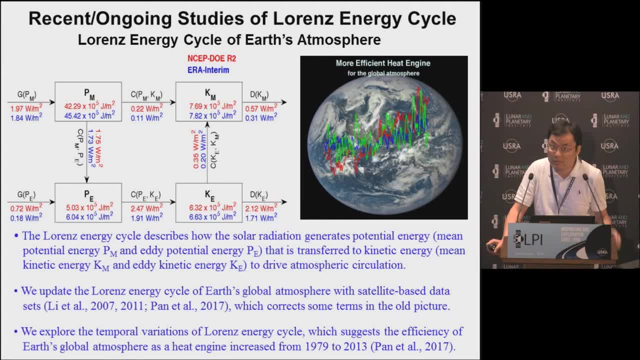 a method to understand the planetary atmosphere from a mechanical energy perspective. so it describes a process in which solar flux generates potential energy, then the potential energy changes to kinetic energy. they interact with the circulation, something like that. anyway, here is for earth results, the previous results based on very limited observations. right here we have more than time. we 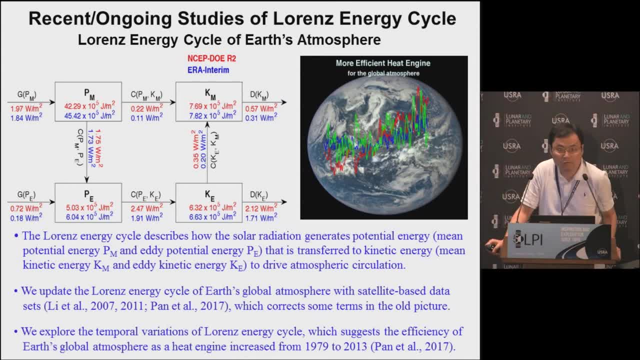 have satellite observations. so we double check the big picture of the energy cycle for earth. right here you have new values. if you compare the new picture with the old picture you can find some times is the old picture. it's not correct. also we double check the global energy. 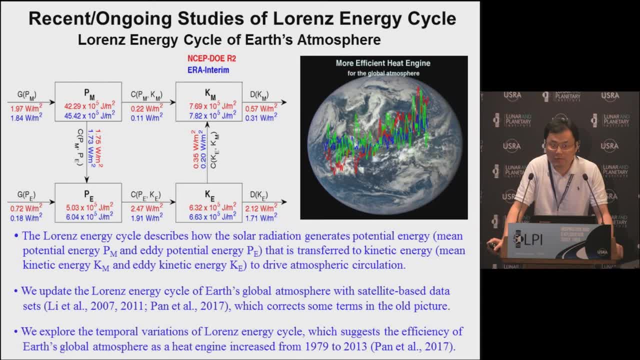 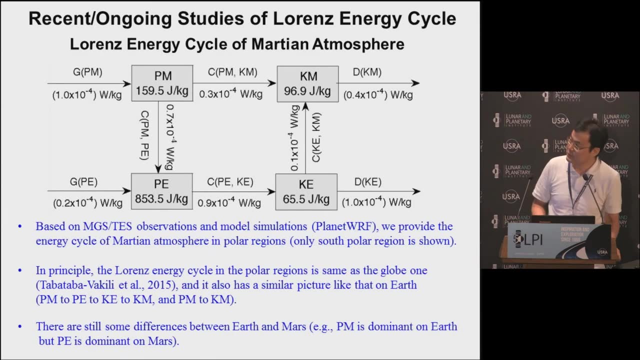 global energy limits. energy cycle for earth. we find, if we take earth, global atmosphere, as a heat engine, actually its efficiency increased in the past 35 years. so we published with this paper with my student. okay, therefore, that's for earth, here is for mars. we double check. 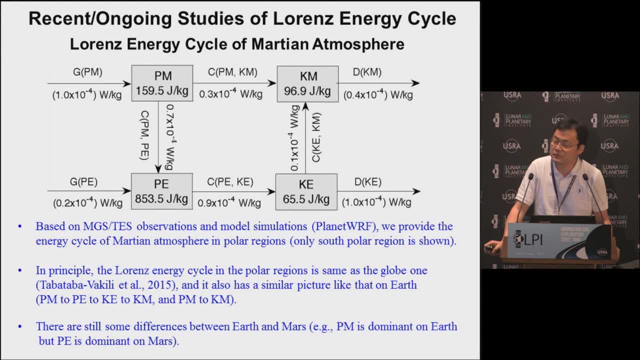 the Lorentz energy cycle of Mars atmosphere. we find basically the Lorentz energy cycle of Mars atmosphere is like that of Earth atmosphere, but still you can find some difference. For example, for Earth the mean potential energy is dominant, but for Earth but for 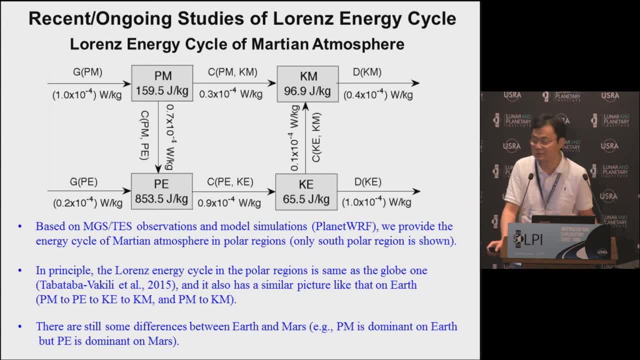 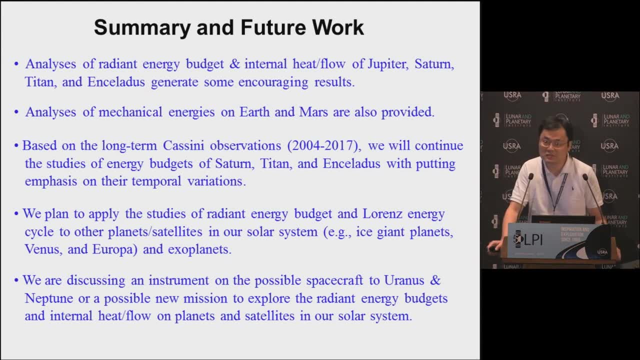 Mars, 80 potential energy is dominant. still some difference between the two planets. Okay, here's the conclusion. I think we provide some studies, recent studies for the- you know reading the energy budgets of the Lorentz energy cycle. so we hope we can apply the studies to other planets and 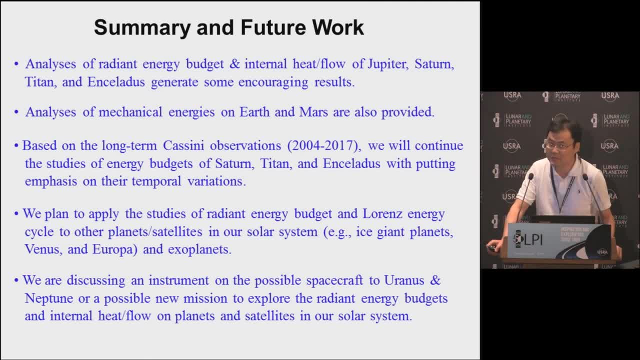 satellites in our solar system. It's also possible to apply our studies to exoplanets Also. we are discussing an instrument or maybe a possible mission to observe some planets and satellites in our solar system. The reason is because of the current observations, The observations of some planets and satellites are not good- not good for the studies of. 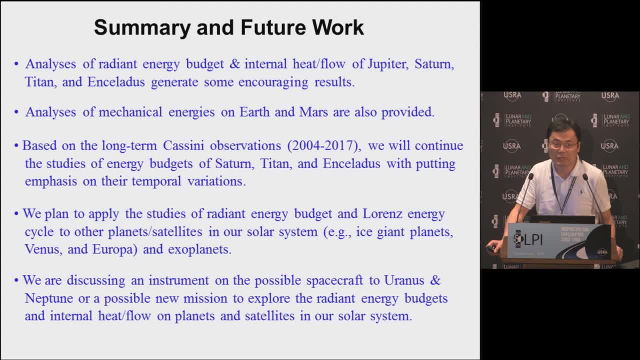 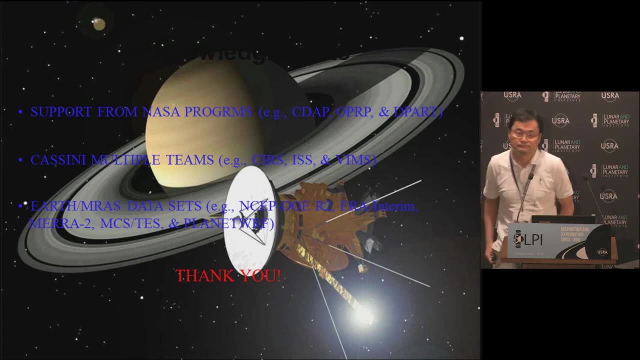 reading the energy budgets. So we think maybe we should develop a new instrument, a new mission to study the reading the energy budgets for some planets and satellites. I think that's it, Thank you. We have a couple minutes for questions, Mm-hmm. 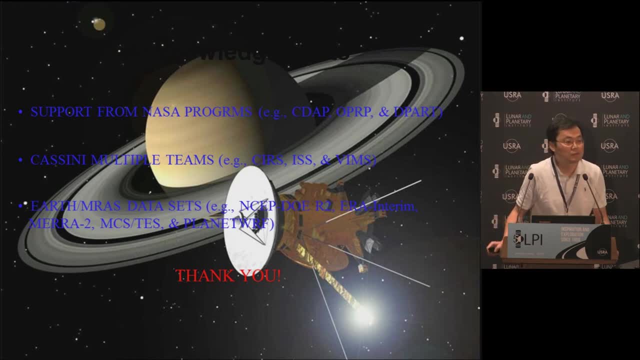 Okay, What data is used to calculate the Lorentz cycle? is it based on GCM simulation? No, based on actually the satellite observations, because, you are right, for the to calculate the Lorentz energy cycle you need a lot of variables. 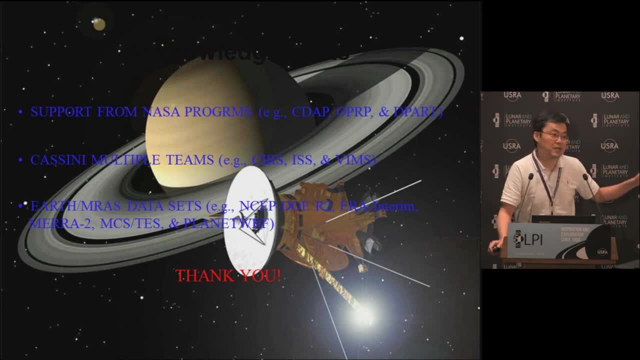 Basically, I think, most of the variables from observations like the zonal wing, like the temperature, the pressure, height. but for some variables like the vertical velocity, it's not easy to measure it, So we use sort of a simulation of the GCM, something like that. but basically it's based. 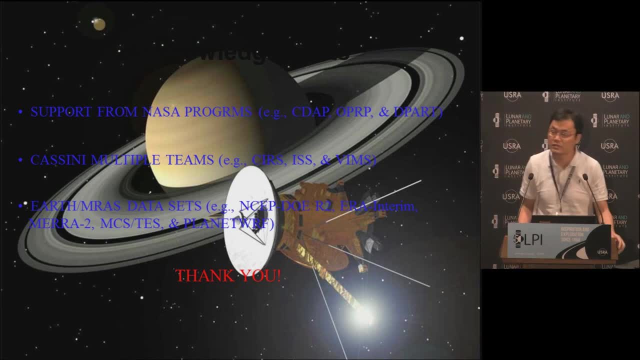 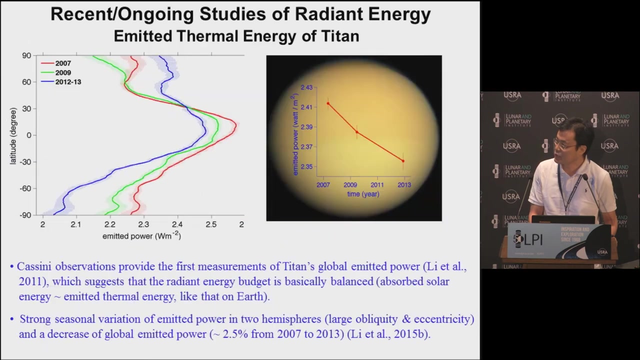 around the observation, not a lot of the numerical simulations. Okay, How do you estimate the uncertainties in the quantities you reported for Jupiter, like the Bond albedo, for example? Yeah, actually, oh, I'm sorry, I put a reference right here. 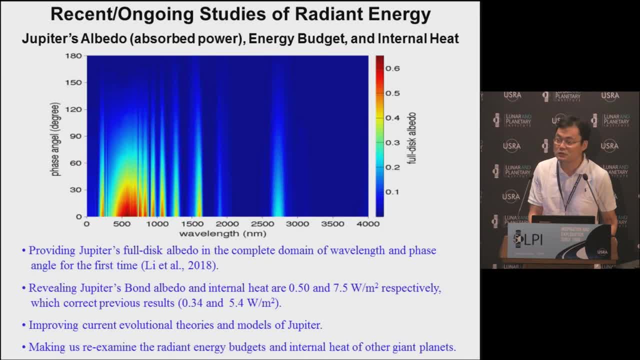 I have a long discussion for the albedo Right. Of course there are a lot of, you know, uncertainty sources. you know, like the calibration navigation, whatever. I put a reference right here. If you are interested you can email me. I can email you back. 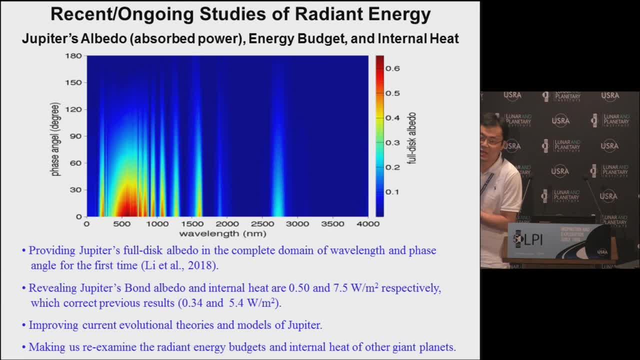 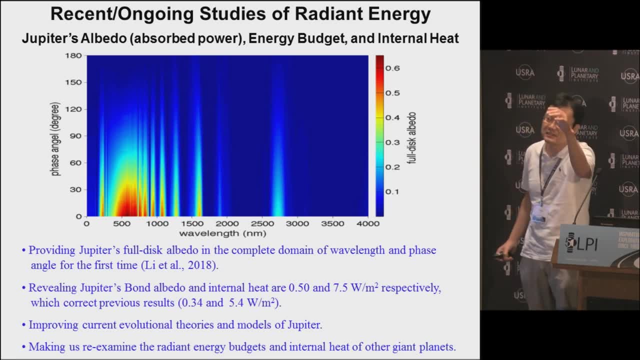 It's in press, not published yet, but it will be published in the next couple of weeks. But anyway, if you email me, I email you back with the reference. I will have a long discussion for all sources, the uncertainty. Actually I didn't put an error bar right here, but actually there is an error bar over there. 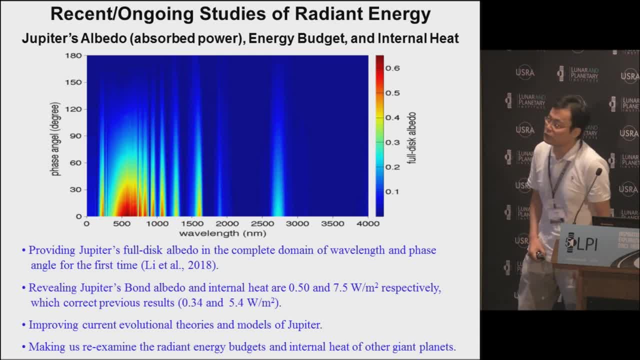 Okay, Is it like 10%? No, 1% at most, Because, as I said, the Cassini observations are basically perfect. The wavelength coverage, the face angle coverage is perfect, basically. So we have very good, I think, results, very precise results, I think.